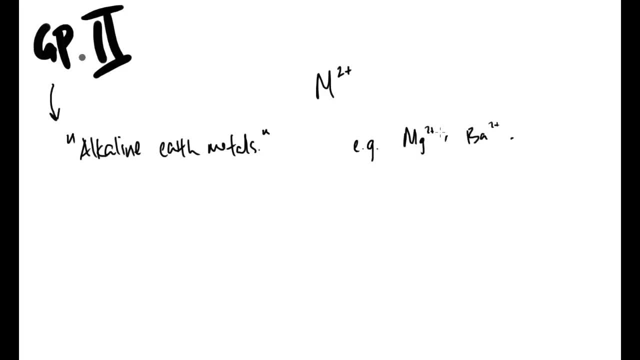 So we've got those ions being made. There's a few points really that kind of it looks at, But it's relatively straightforward actually the whole of this topic And it's very, very small actually And one that I think people sometimes get themselves a bit too worked up over. 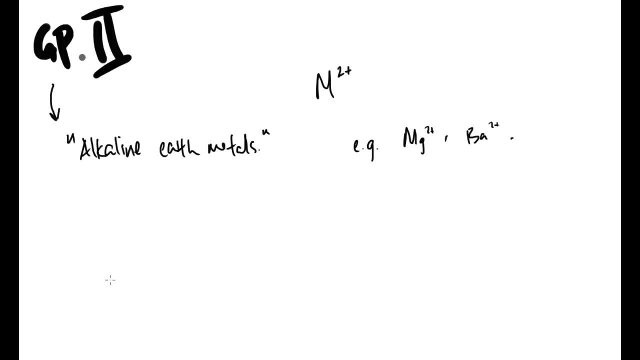 There's not a lot of scope for questions being asked. So, first of all, how do they react? Well, they react with water, So react with H2O, And they all react in a very, very similar way. And if we just use again this generic M to represent any of the metals, 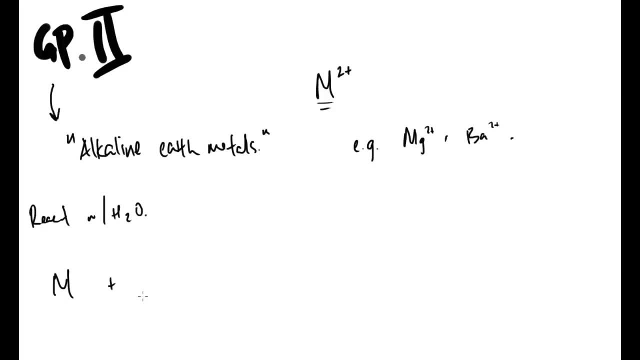 They react as in ionic terms they react M And they go look at this And they become the M2 plus ion. Add two electrons. balance that out by that half equation As they're forming this M2 plus ion over here. 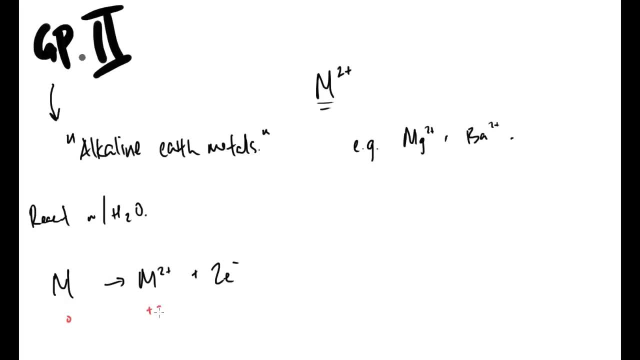 And if we look at oxidation state terms, we can see we go from 0 to plus 2.. Therefore there is an oxidation occurring in this situation. So we've got oxidation. So they're oxidized. when they react, They lose electrons. 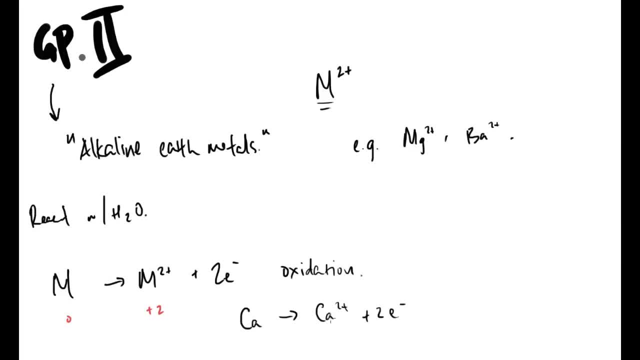 Example. I'll give you an actual sort of a proper one here. Ca goes to Ca2 plus plus 2 electrons. So a reasonably sort of straightforward thing, Just substituting in our elements our group 2 elements for the letter M here. 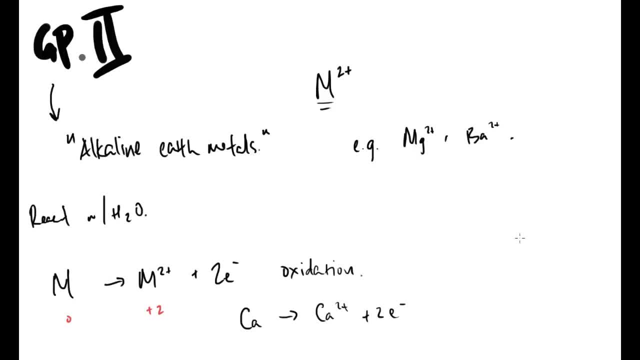 Which makes it quite easy The actual go into a bit more sort of detail actually about the reaction with water. So that's their. the way they react is like this: But the actual reaction with water, more specifically, is that our metal, again using this M. 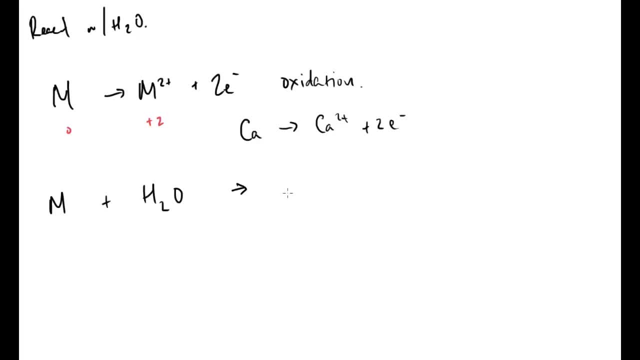 It reacts with oxygen, The water, to form specifically the hydroxide, And that's a very, very important thing. So we'll use this again: generic M and we'll go across here and forming hydrogen there. So M plus water gives us MOH2 plus H2.. 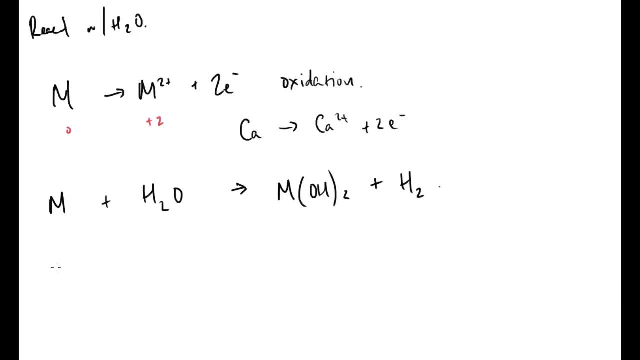 And all you have to do is substitute in the M for the element that we're dealing with. So we'll do magnesium, for example. So the magnesium, we will react that And with the water to form magnesium hydroxide and hydrogen. 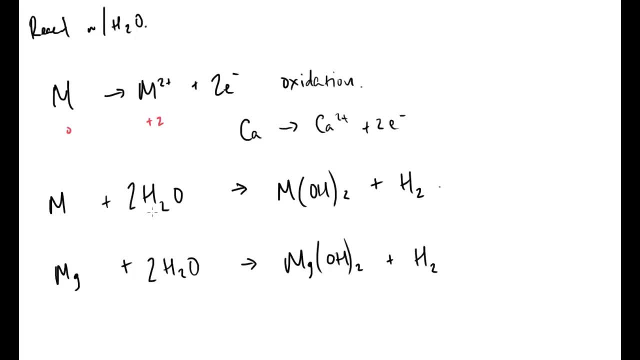 And of course, we must remember to balance things. We have to obviously have balance there To make sure obviously, our hydrogens and our oxygens are balanced. The one key thing here this is if we use state symbols here. 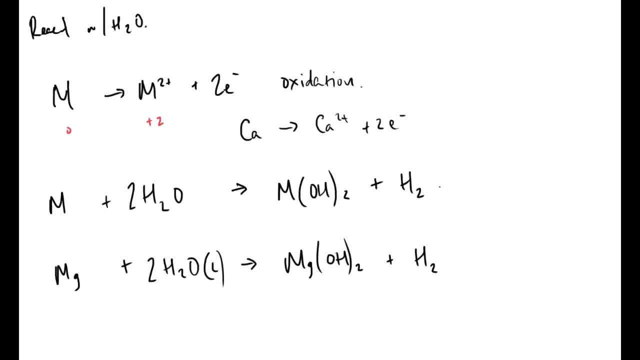 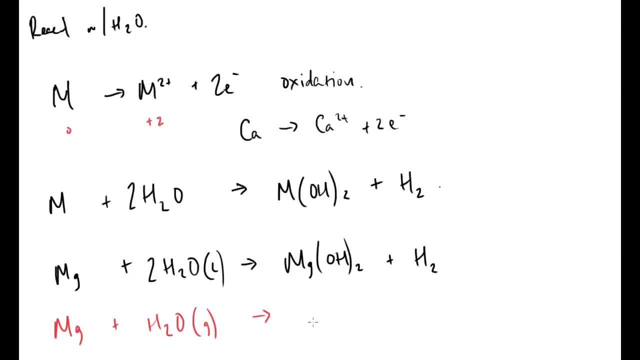 So magnesium reacting with steam, So magnesium reacting with steam. Steam, again still H2O, but in a gaseous state actually forms the oxide and then still H2.. So that's a point to really be aware of. is that you could be asked either of those? 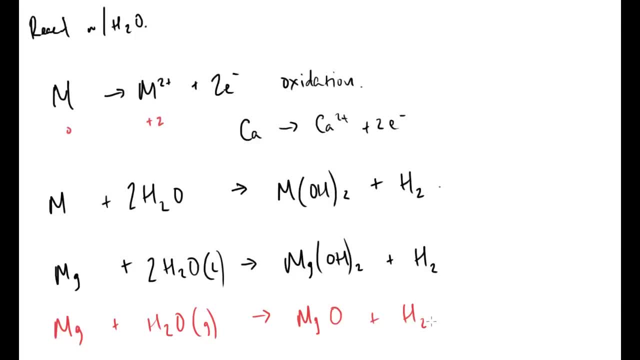 And it's just a very small thing, But again that might get you another mark, two marks in the exam or probably a mark actually, But it's still. that's a mark that you know could be the difference between sort of an A and a B. 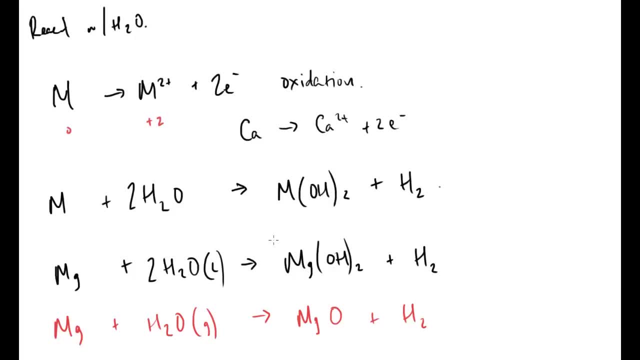 C and a, D or whatever. So point there to note reactions with water, reasonably straightforward If we look actually at these reactions as well, and I will touch now very quickly on the reactivity If we go down group two. so start at the top with beryllium going down to barium. 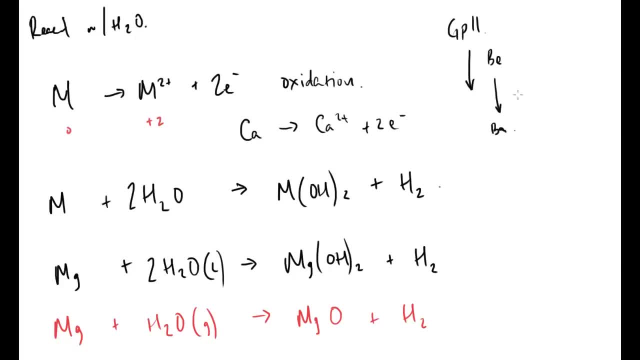 we'll find that, generally speaking, the reaction increases, So the reactivity. So the reactivity Increases. And if you think about this in terms of the reason why that happens, well, as we go down, it becomes increasingly easy to oxidize our atom into the ion. 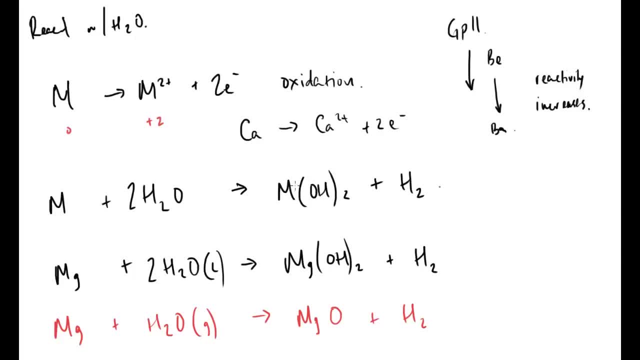 And that's really what's happening here. We're going from atom to ion here. So magnesium, for example, going from magnesium atom to magnesium ion within the magnesium hydroxide, And so because as we go down the group, the atom gets bigger, those outer electrons are further away. 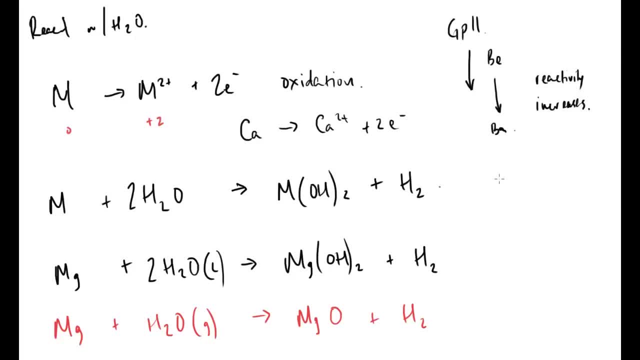 And so removing them becomes easy because there's more shielding and there's less, therefore less attraction to the nucleus. It's further away and more shielding, easier to remove them, therefore more reactive. It's the same reason for the group one metals to go down. 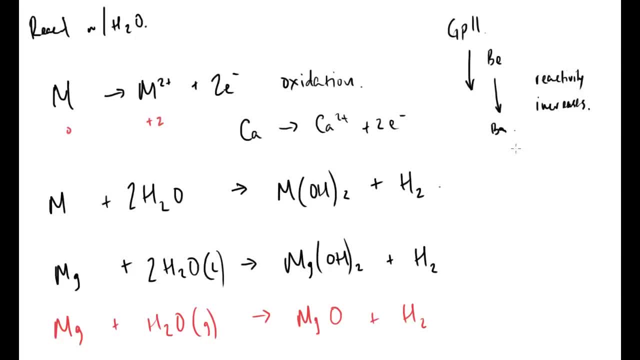 That's a very obvious one. we see- And actually you can see this kind of thing in class- If you take something like calcium, certainly calcium with water, it's quite a vigorous reaction actually. It's, it's, it's. it gets very hot. 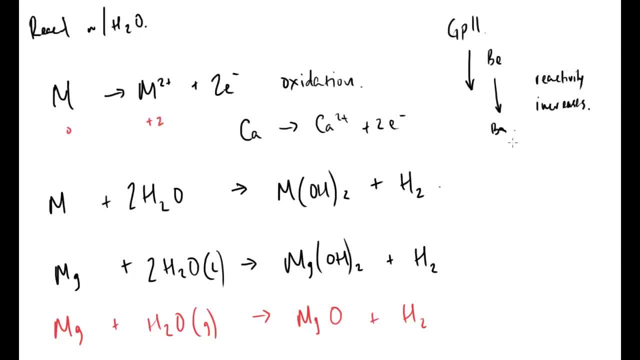 Magnesium. Magnesium is is slower but still occurs And obviously, going down towards barium, it's a very, very rapid, very rapid reaction indeed. So this is a bit about the reaction with water. Take into account here this special case of magnesium reacting with the steam. 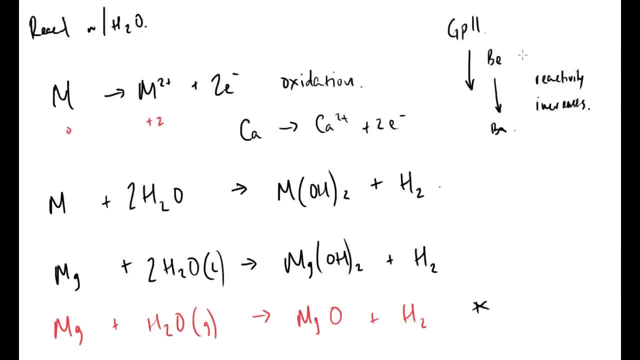 A bit disjointed here. Beryllium, no reaction. Okay, I should really mention that, but I think in the exam I can't imagine them asking you to write the equation for a beryllium- Okay, A beryllium reacting with water, and it being a trick to say, oh, there is no reaction. 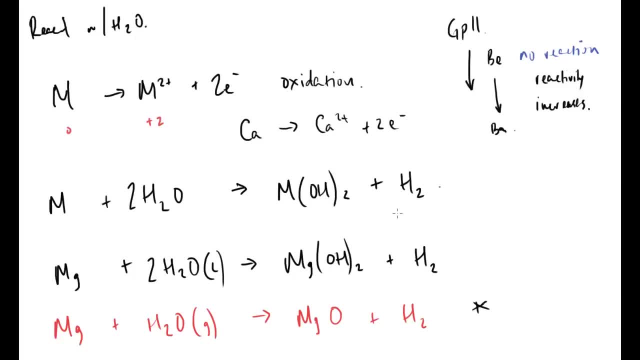 Normally they'll specify: oh, write the equation for magnesium with water, Magnesium with steam, beryllium with water, they said. Or maybe write the ionic equation, in which case you would just be dealing with this guy here. 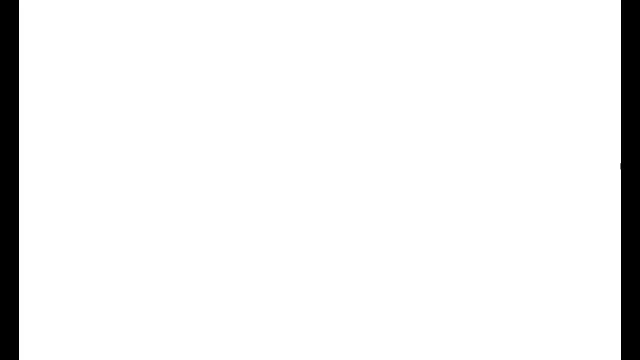 Okay, going down, looking a bit at the next section, which is in group two, which is the solubility of a compound. This sort of plays itself into the solubility of two specific compounds. Look at the solubility of the hydroxide. 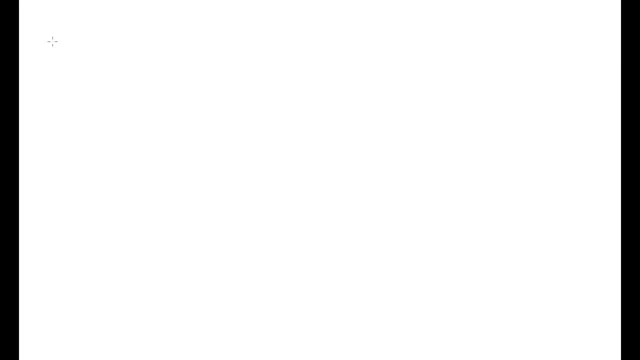 And look at the solubility of the sulfate And the easiest way to do this- just think about it- going down the group, So going down the hydroxide versus the sulfate. So this is going to be least soluble, going to most soluble. 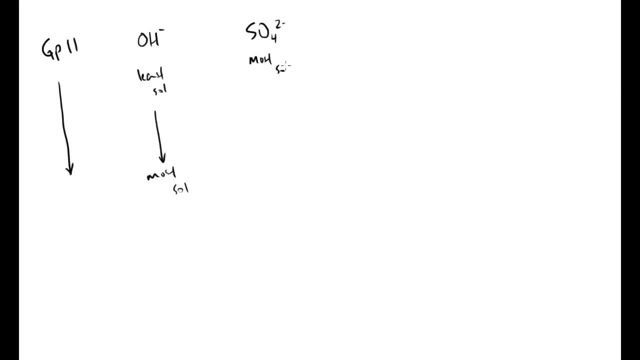 This is going to be the complete opposite: Most soluble To least soluble. So, for example, magnesium hydroxide is going to be very- it's practically- insoluble. So actually that forms precipitate Magnesium sulfate. on the other hand, MgSO4, that's going to form a nice solution. 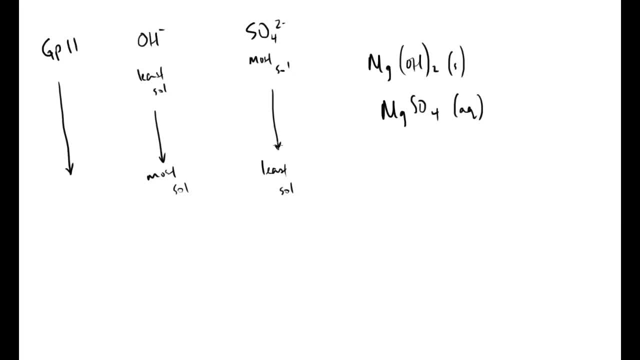 And the question will guide you around what they want there. They're not just going to specifically ask you to explain a trend. They will give you variance. They will lead you into various sort of alleyways with what they're questioning you. The key thing is they can link into here. 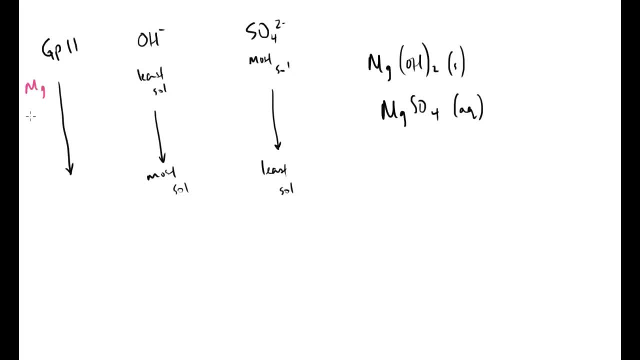 So if we start up here at the top specifically, we're looking at magnesium, going to calcium, to strontium and then to barium. This tends to be one that they love talking about. So this idea of least soluble up here, 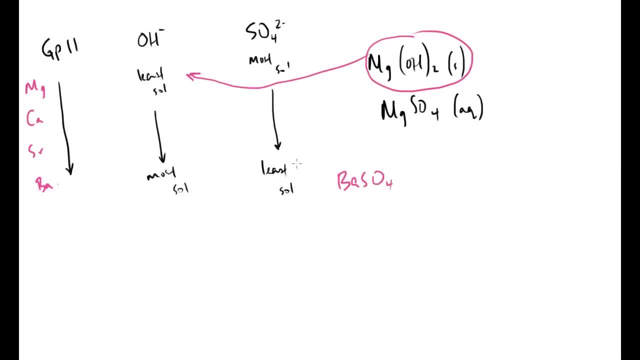 And the barium sulfate that we produce here. they love to talk about this one as well. So the magnesium sulfate, Magnesium hydroxide, They like questions like: well, what could you use magnesium hydroxide for? What can you do with this? 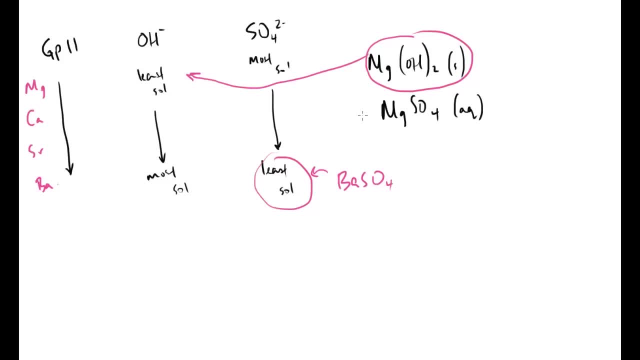 Blah, blah, blah, blah blah, And actually it's one of those quite nice ones in that you can use magnesium hydroxide as things like different color for this, so it can stand out. antacids, And what I mean by that is really indigestion tablets. 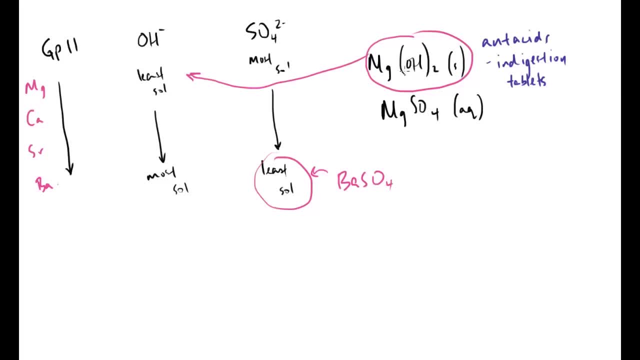 That's a key reason. You wouldn't normally want to be taking a hydroxide Orally. you wouldn't want to drink sodium hydroxide, for example, Because the magnesium hydroxide is a solid. there's not really a risk there, okay. 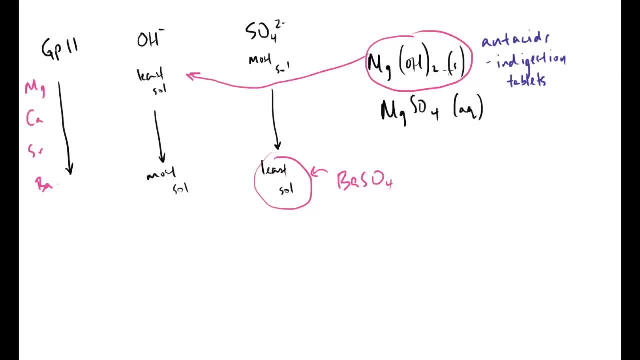 And that's because it's a solid. It's insoluble, Therefore it's not going to cause that damage. It doesn't act like a normal alkali. That's a very key point. The other way they like to look at these various parts is, as I said, is with this barium sulfate. 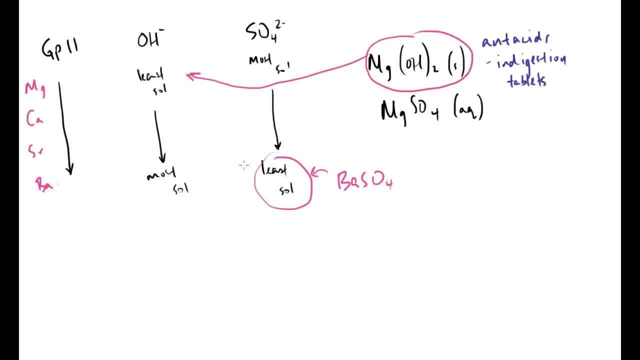 And I'll come on to a second, a bit more about this, and there's a test that you can look at, But barium sulfate. While we're talking about this, we're going to talk a little bit more about barium sulfate. 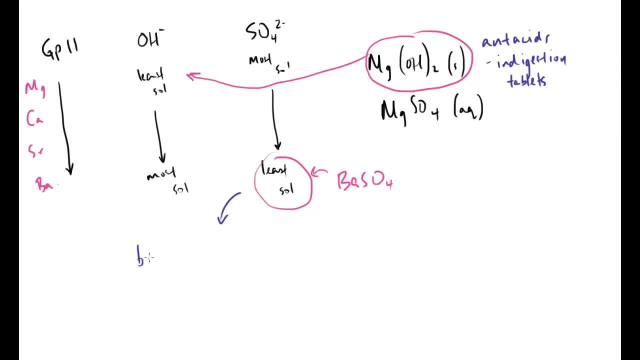 And we're talking about sort of uses for things. Barium sulfate is used as what's called a barium meal, And a barium meal is something that's given in hospitals when someone is going to have an x-ray, Or particularly an x-ray of their GI tract. 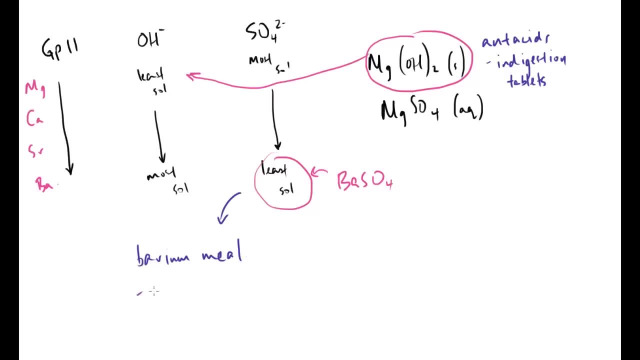 So the intestine and all that area, And the reason is that the barium meal, the barium sulfate, absorbs the x-ray. It's brilliant, So it's. it actually finds that it, so it sits in your indigestion, indigestion, it sits in your digestive tract. 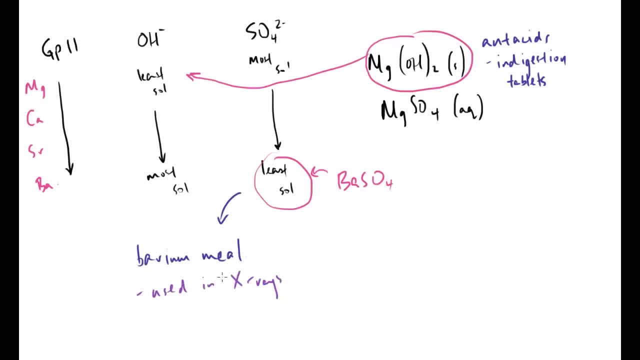 And what it does is it'll absorb the, absorb the x-rays, And so it allows for doctors to basically see, kind of, if there are any problems with that in you know intestine or the stomach or all the rest, Because you can see very clearly it shows up actually. here's a picture: 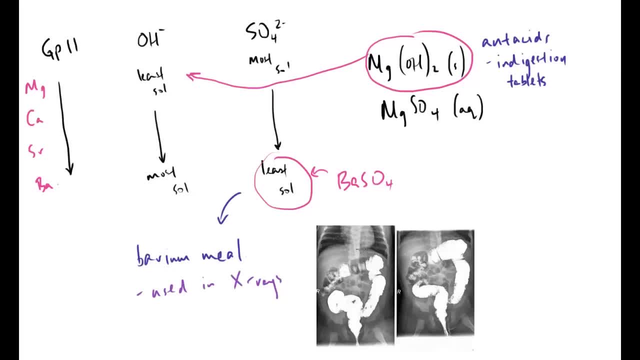 This is what it kind of looks like on a, on a, on an x-ray, And so you can see here actually what's happened is the person has swallowed The, the barium meal, And you can see what's happening is it shows up very clearly white hair. 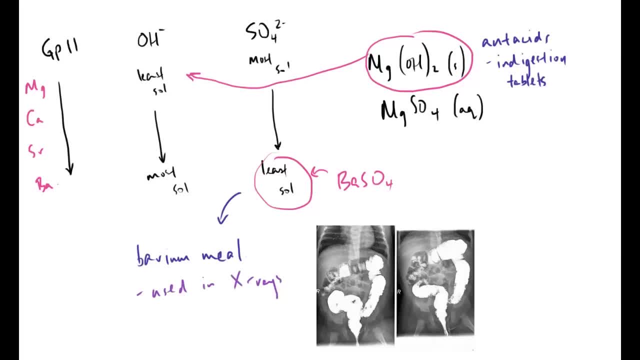 Now, I'm not a doctor, so I don't know if this person has any problems with them or not, but obviously, hopefully not. But you can certainly see the barium sulfate showing up Now. there's another reason for using the barium sulfate. 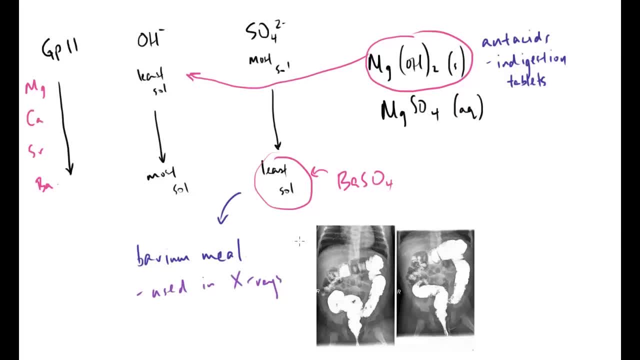 It absorbs these, these x-rays, brilliantly. Well, not another reason for using it, but another quirk of of question they'd like to ask, And that's that barium tox, barium, barium toxic, barium compounds are basically toxic. 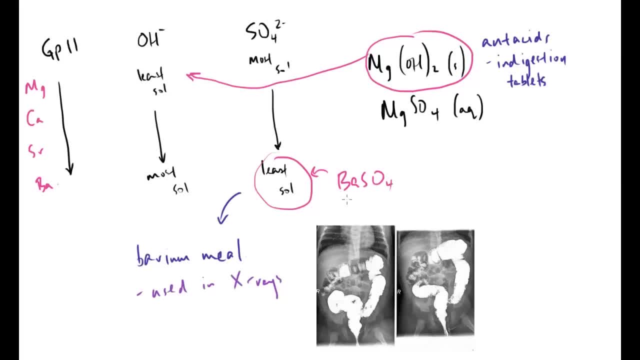 And the thing they look like. What they love to ask is: well, if barium's toxic, how come something like a barium meal can be used, can be swallowed, can be taken orally? The reason is that it's not soluble. 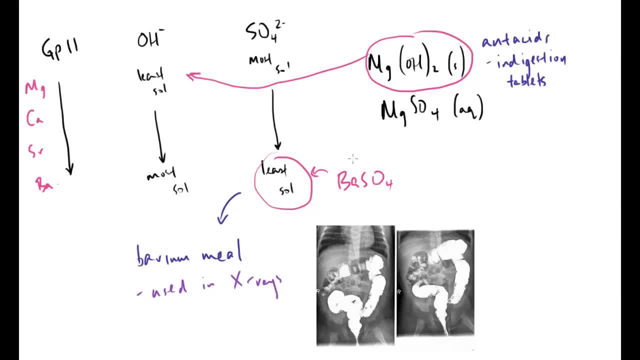 It's not soluble, so therefore the barium doesn't actually get into the body. It's taken it through the mouth. It works well and it goes out here and we don't have to worry about it anymore. So it comes in, it goes out. 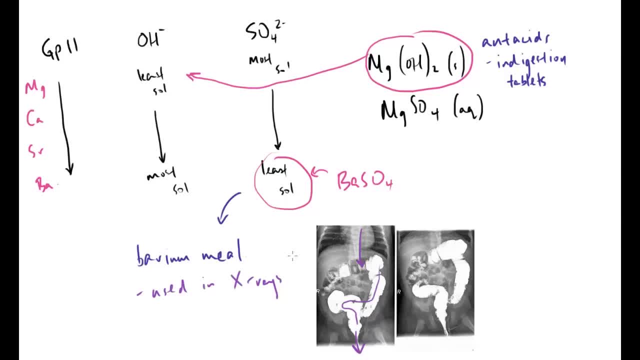 There's no toxic nature to the body and that's because it is insoluble, So actually, least soluble, yeah, it's actually insoluble. okay, So it would be a solid, does not dissolve and therefore provides no risk when taking it as a as a suspension, as this barium meal. so that's absolutely fine. 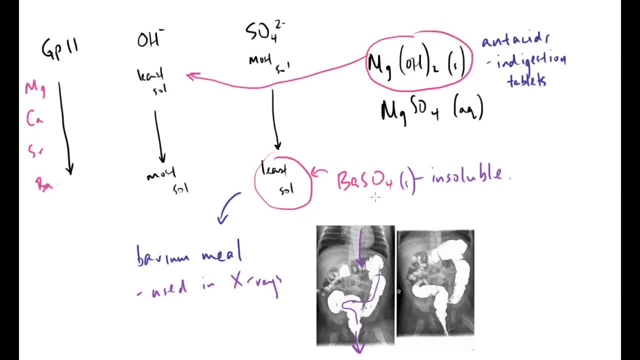 The other uses of things that you might come across. calcium hydroxide is particularly used. it has another name, it's called slate lime, So I'll put this. I'll choose a slightly different colour, run out of colours here, So CaOH2.. 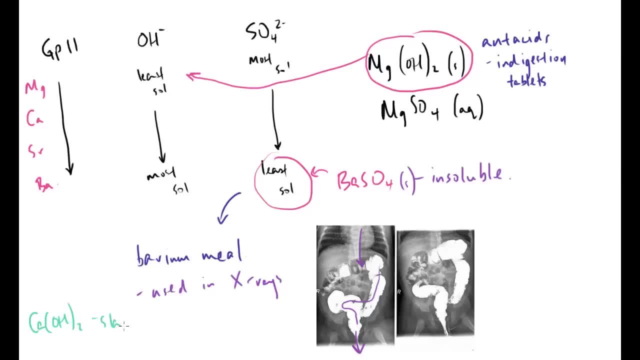 CaOH2.. CaOH2.. CaOH2., CaOH2.. CaOH2.. Slaked lime and this is used on fields. really, it's used as neutralising- neutralising acidic soil, and it's a fairly inexpensive way of of reducing the acidity and allowing crops to grow, basically, which is obviously quite important for farmers and all the rest of it. 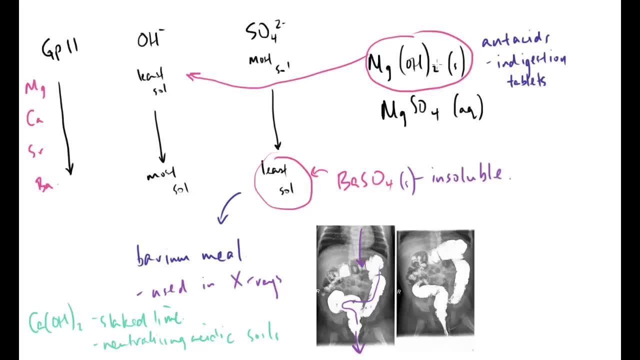 And that's really uses done so, specifically the ones that have come up in the past on papers: magnesium hydroxide, calcium hydroxide may have done, but barium sulphate certainly does, as this barium meal, And that's really uses done so specifically the ones that have come up in the past on papers. magnesium hydroxide certainly does as this barium meal. And that's really uses done so, specifically the ones that have come up in the past on papers. magnesium hydroxide certainly does as this barium meal And that's really uses done so specifically the ones that have come up in the past on papers. magnesium hydroxide certainly does as this barium meal.